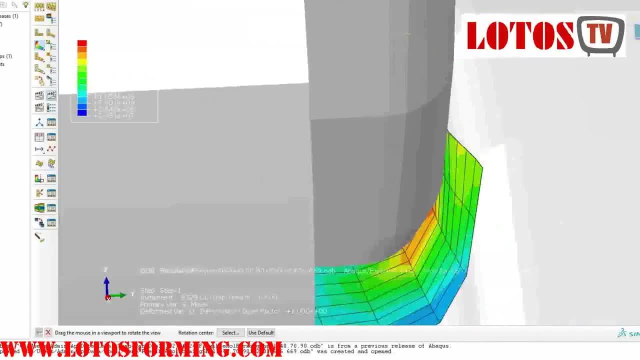 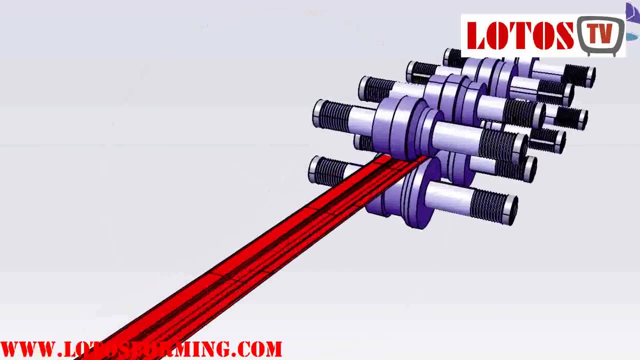 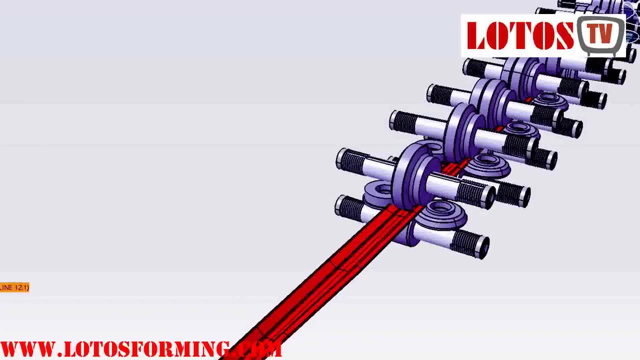 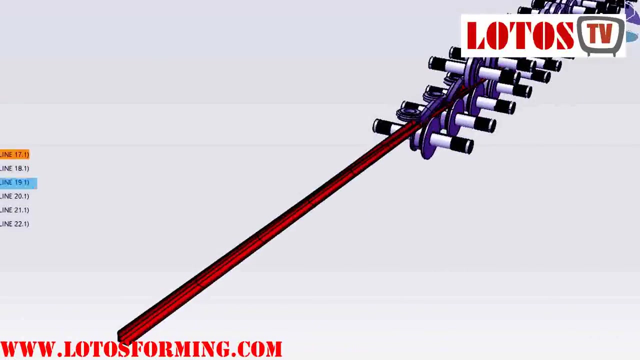 this is the roll forming machine we talked about in this video. so one more time again, roll forming is the continuous bending and shaping some sheet metal to some design or demand profile. for any roll forming manufacturer, these days we need a CAD design, computer-aided design for 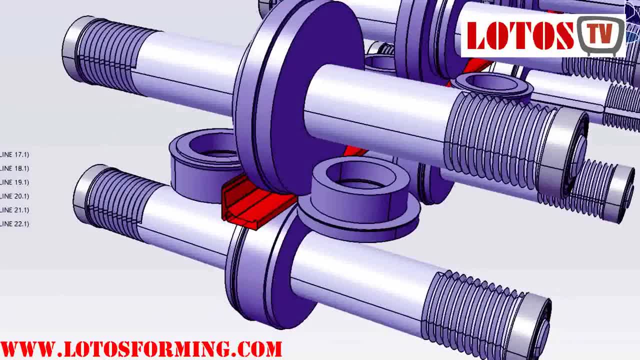 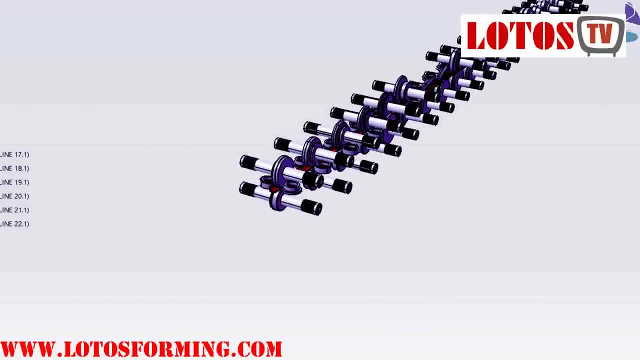 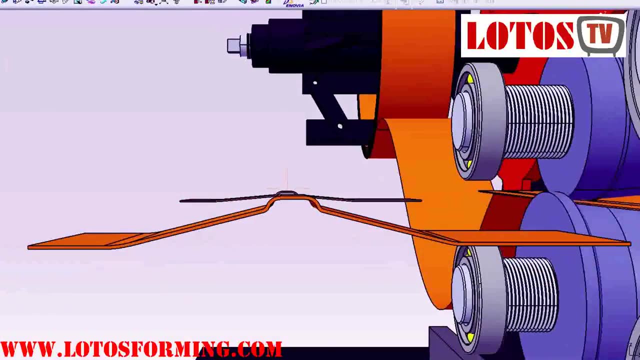 3d design for roller shaft and each part of the machine and also meanwhile we needed some analyzing uh system by abacus or other software that we can analyze these design is working proper or not, as you can see in this video I'm showing you some recently roller and shaft. 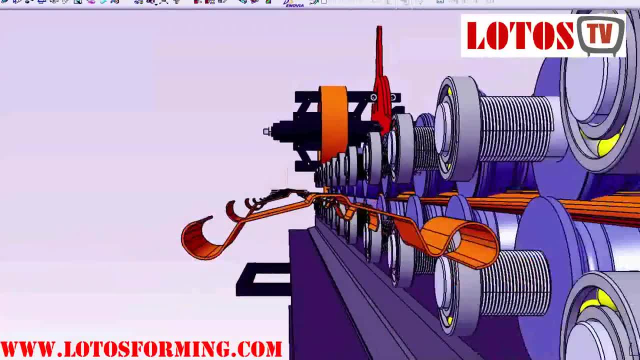 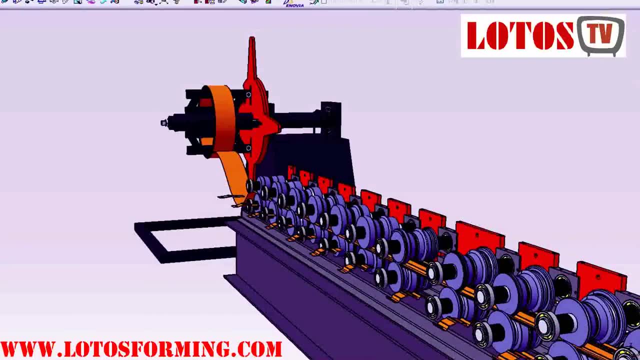 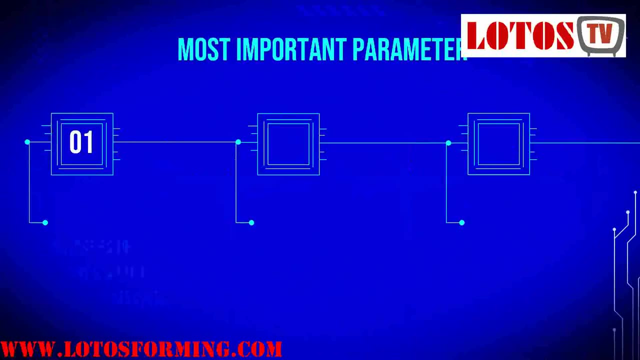 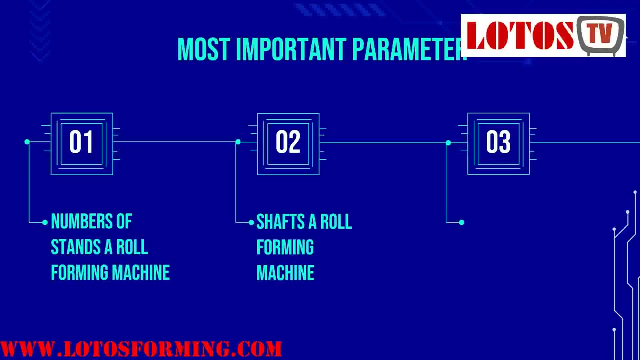 and how it bend and how it changed during our roller continuously. so pay attention. we start from the color and one by one we go ahead. so now I want to talk about most important parameter in roll. forming machine number one is not in stands error. Forming Machine number two is the shaft of your forming machine. 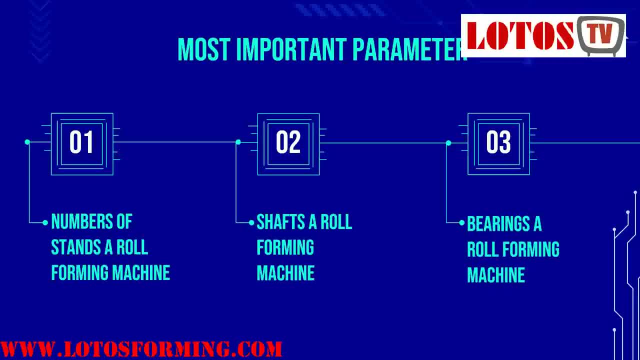 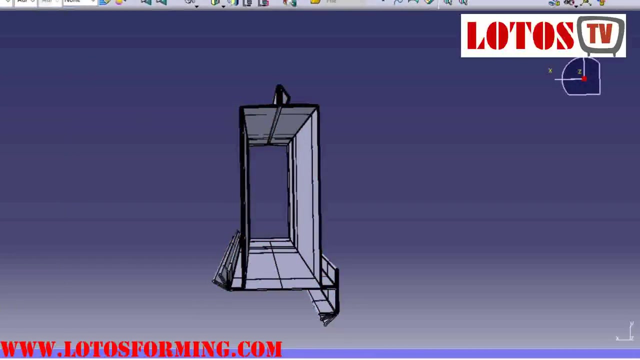 number three is the bearing be used for each shaft. number four: the cleaner of a forming line. number five: structure of stands. number six: material of rolling tools. let's start from the Number One. number one is stands- number of stands roll forming machine. based on the different experience and the different 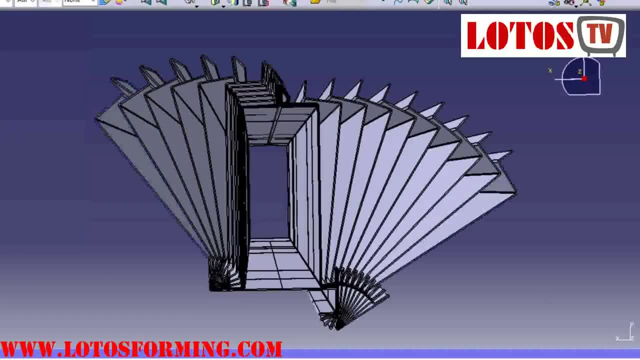 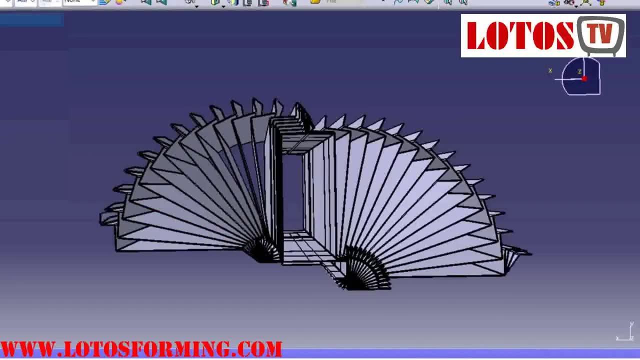 manufacturer in China or in all the world. same profile, same requirement. we use different amount or different quantity of stands generally, once we use less stands, the machine cost will be lower, but it's also effect by your final shape quality. so any shape or any design need a really experience. 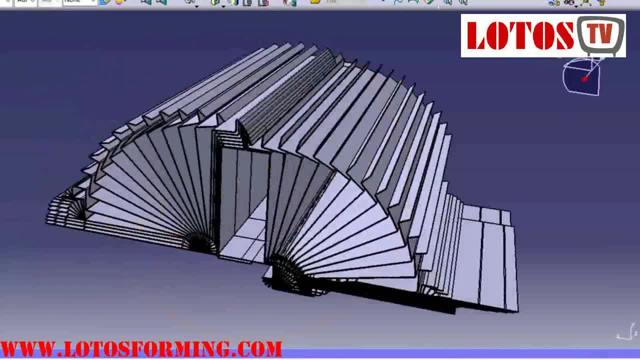 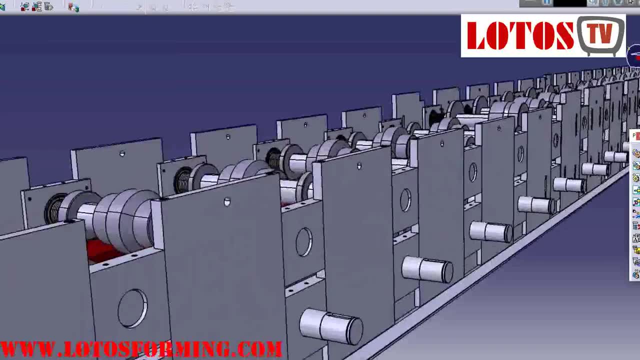 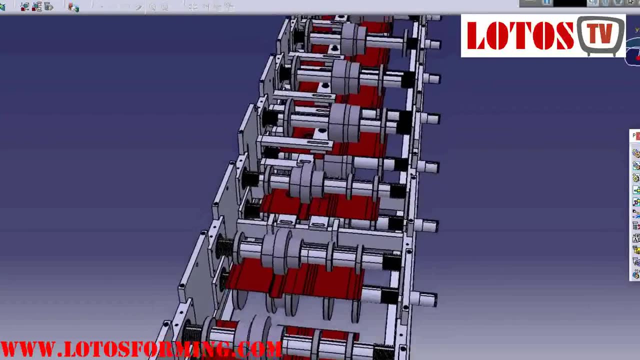 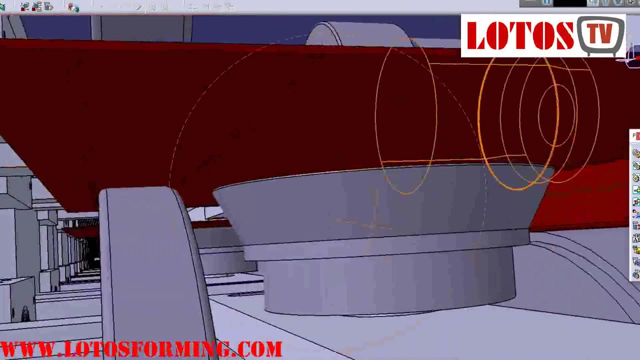 for different design and different manufacturer. we use a different amount of the stands here you can see, or design for one roller and my shaft and this is all final stand before the coming out from machine. so with once we take in the stands or one roll forming stand, we call about down roller, up roller and the shafts. 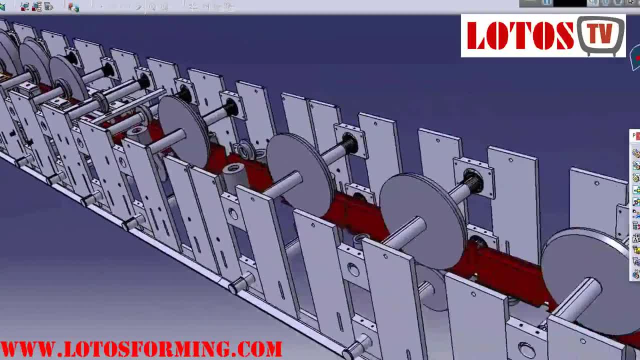 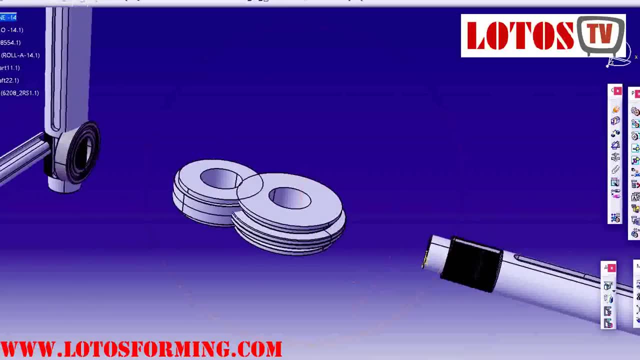 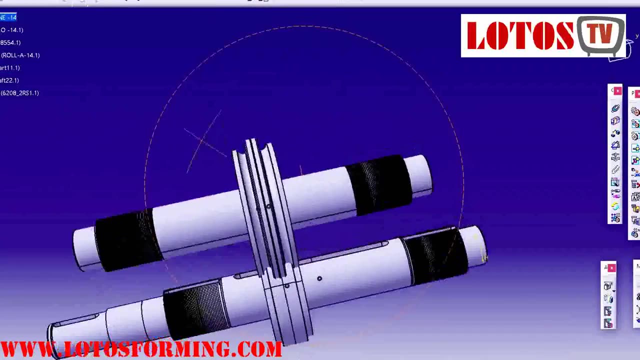 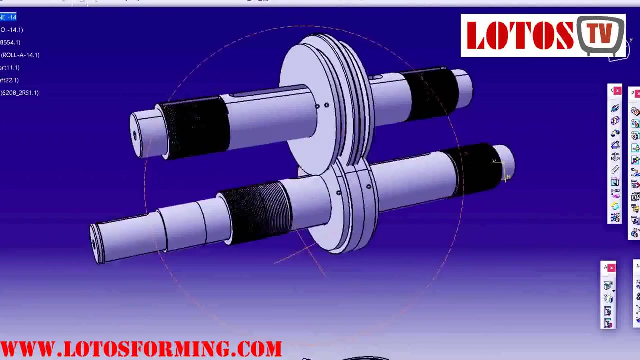 the second item is the shaft. for any stand we need the up roller and down roller shaft, shaft diameter and shaft. the material quality will affect on your price and your quality of profile if the thickness is less than one millimeter and the width is less than 200. 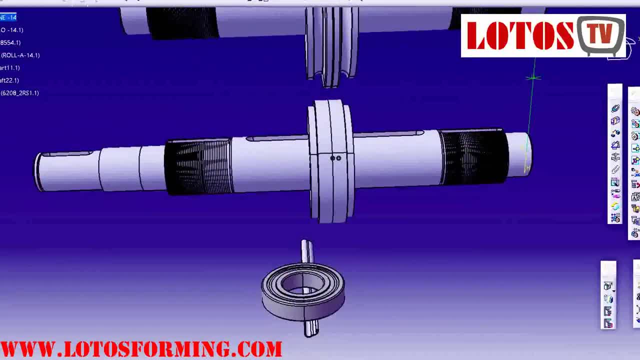 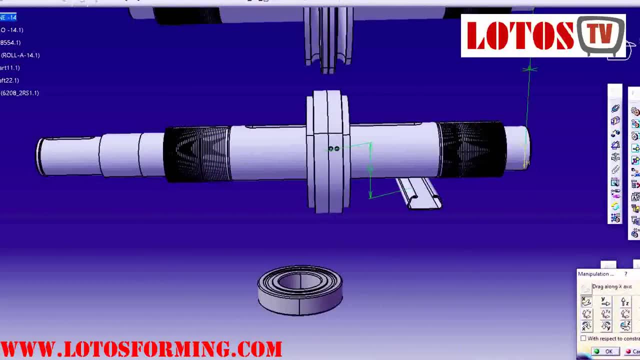 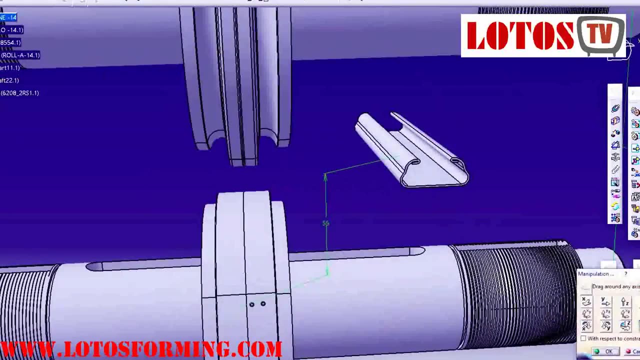 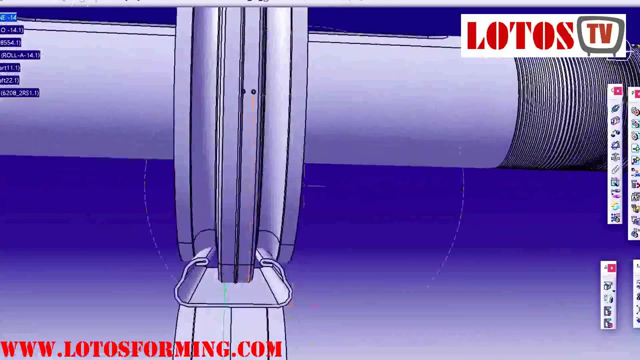 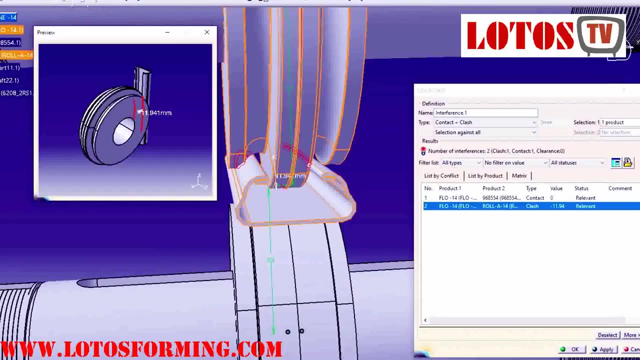 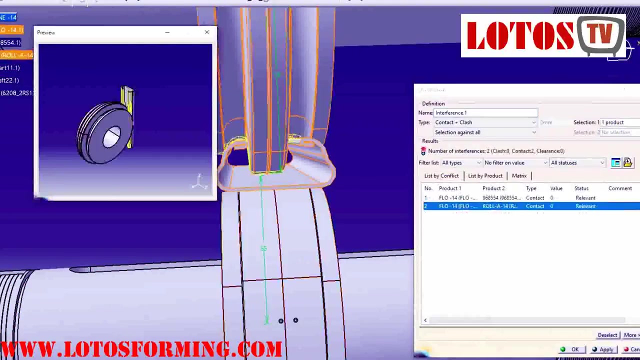 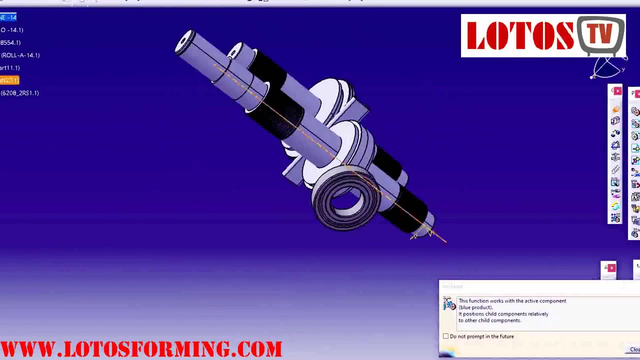 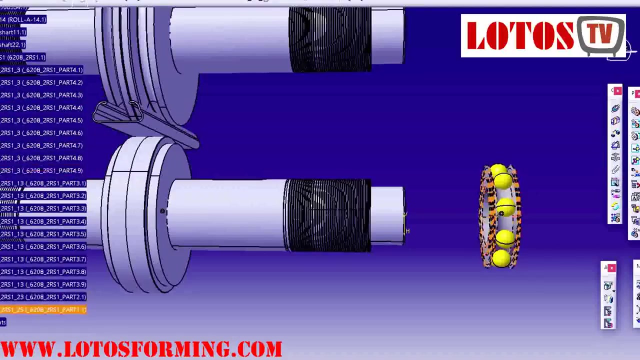 we mostly use a 50 or 60 millimeter diameter and some of them higher than one millimeter. we analyze by software and we apply for higher diameter of shaft. so the diameter of shaft, the material that you use and the machining process is really important. number three: we talking about bearing, performing machine bearing. you know design, we choose and 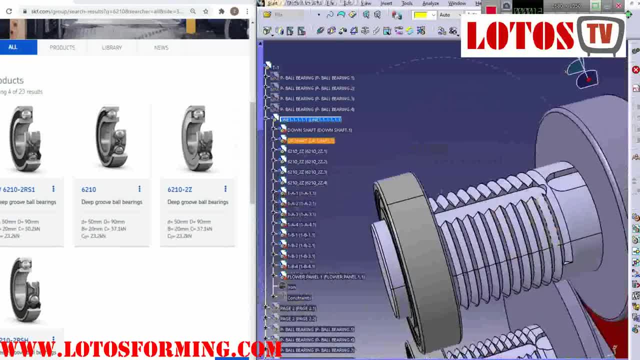 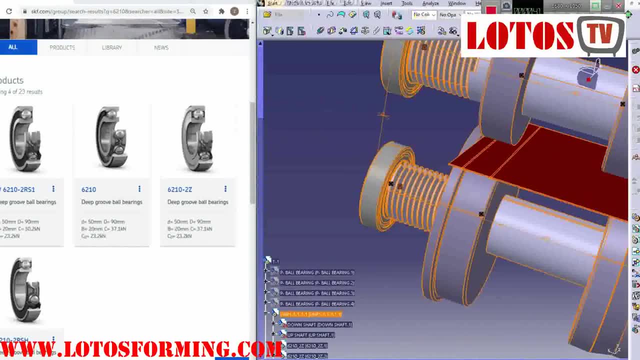 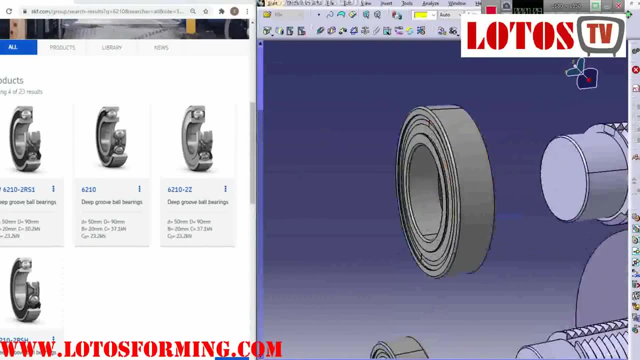 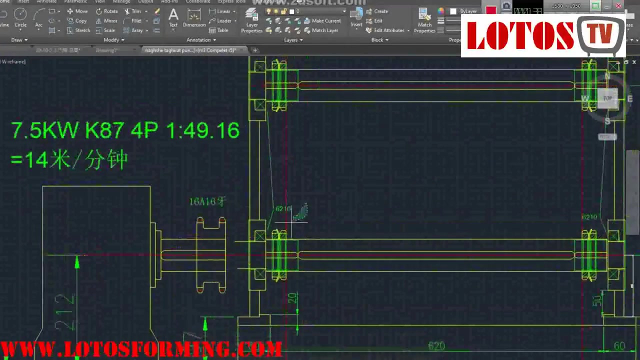 we analyze what kind of these standard of bearing we use and the brand of the brand. in Lotus you mostly using Sky F or NS Cup brand but you can see in China or other countries they may use cheaper brand for lower the cost and lower the price for the customer. but we insist on. 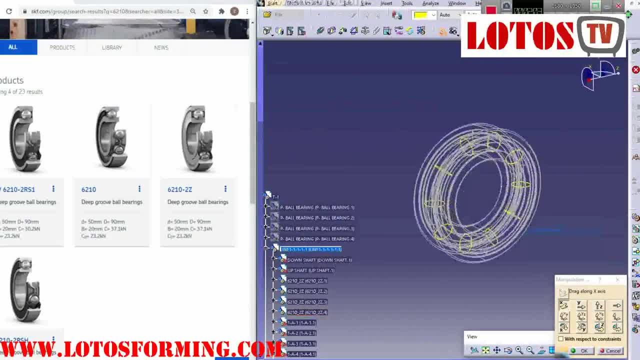 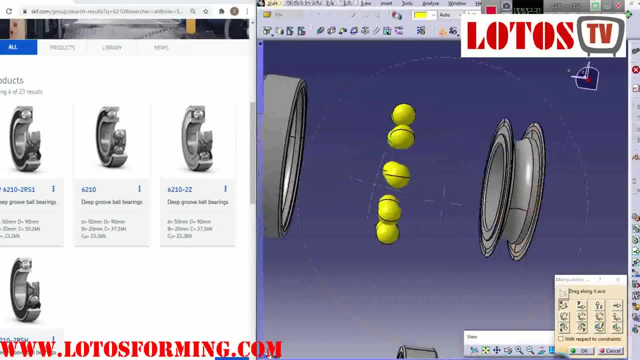 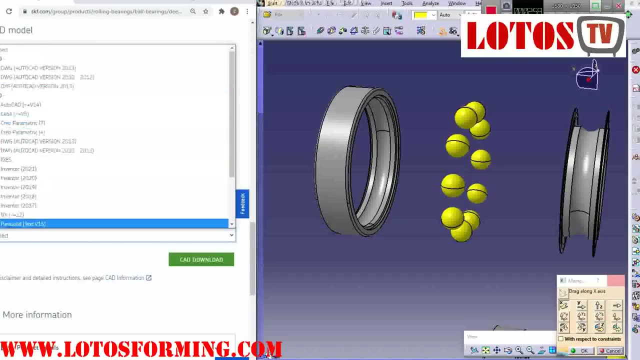 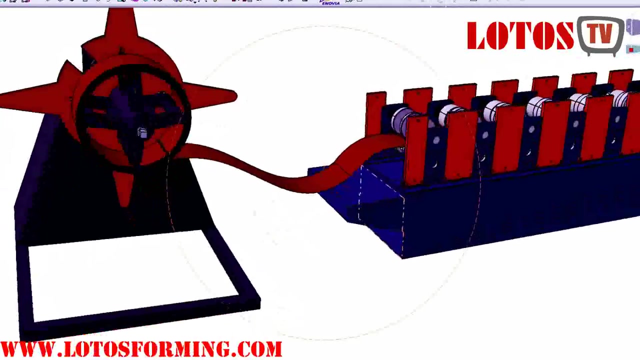 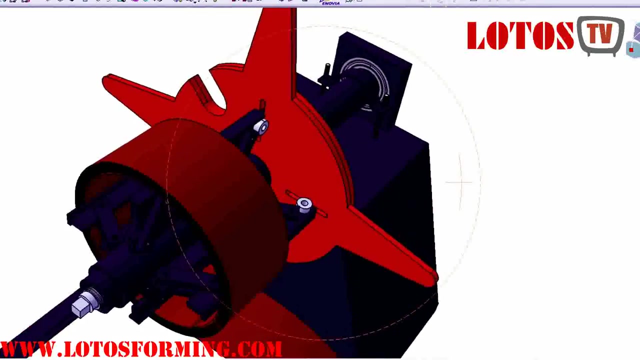 the best quality of the roller and best quality of the bearing because it's effect in the long time. number four: decoiler. for any reforming machine with the manual decoiler or motorized decoiler, we have a different type of decoiler. you can check our page in our website. we have a special page for 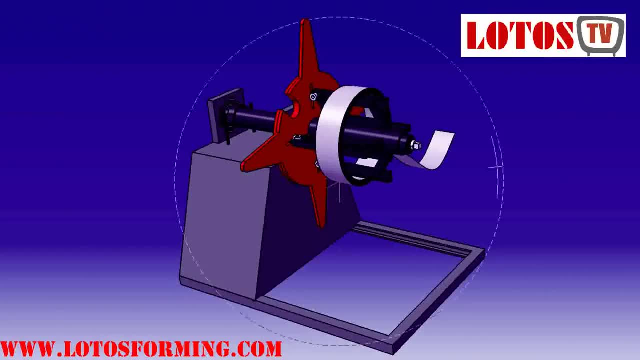 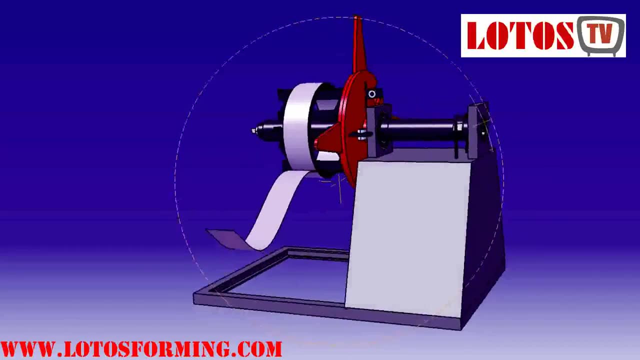 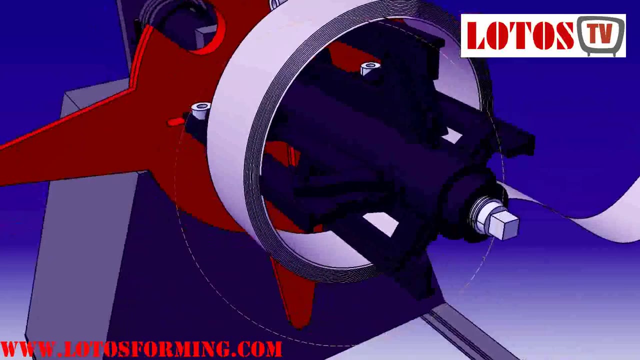 decoiler. decoiler is the some component or some part of the machine that we put coil on, that raw material, coil on that, and we step by step open it and fed through the machine. as you can see, we have a motorized decoiler, we have a hydraulic decoiler, we have a 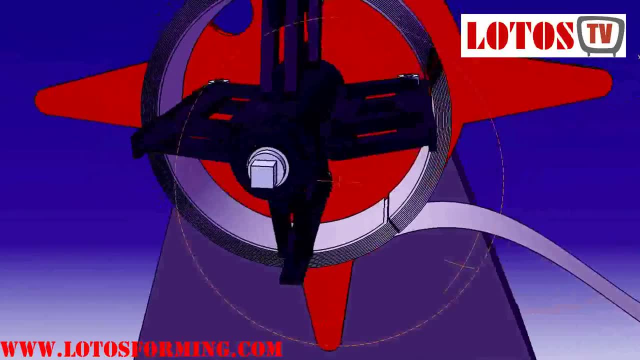 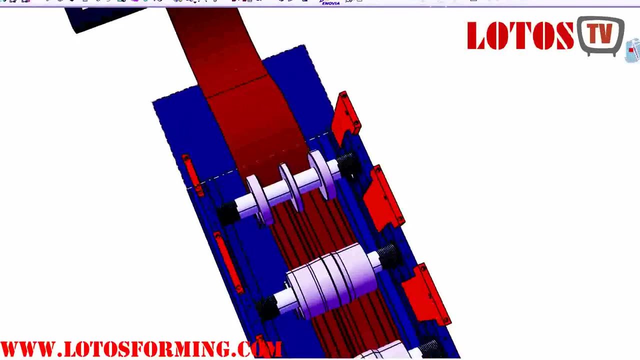 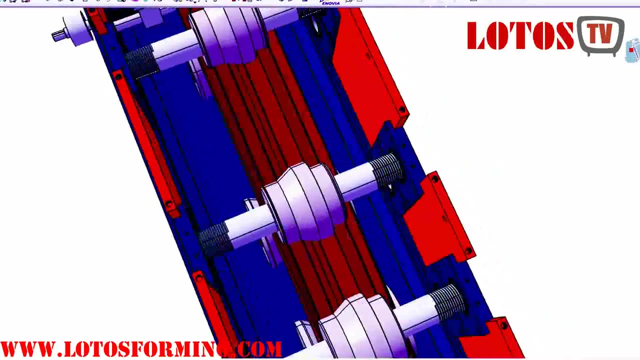 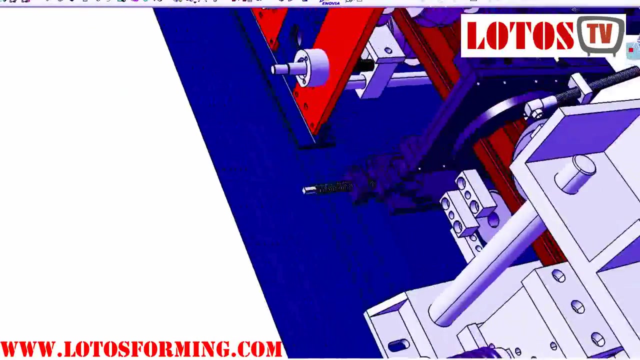 automatic decoiler with the coil card, decoiler without coil card. it's up to your material thickness, material weight and material width. we apply for different decoiler. number five: i want to talk about structure of stands. any manufacturer in the world, or any manufacturer in china, has their own standard for 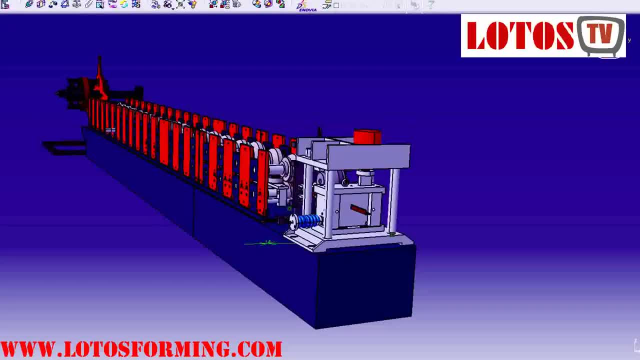 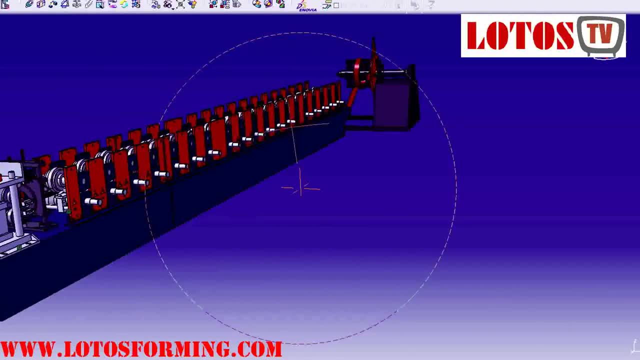 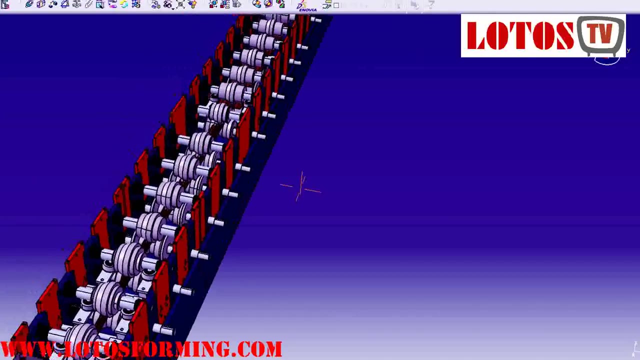 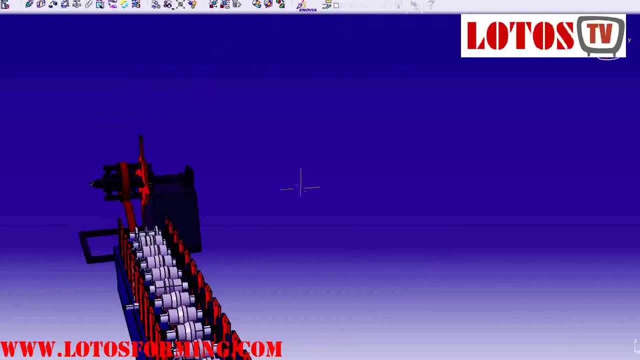 structure, main structure for stands in our lotus. we have a two tape of the stands. one is economic tape and we use a base on a steel sheet machining and a steel sheet milling. that is economic and mostly we use for domestic cheap customers. secondary is the casting plan for the 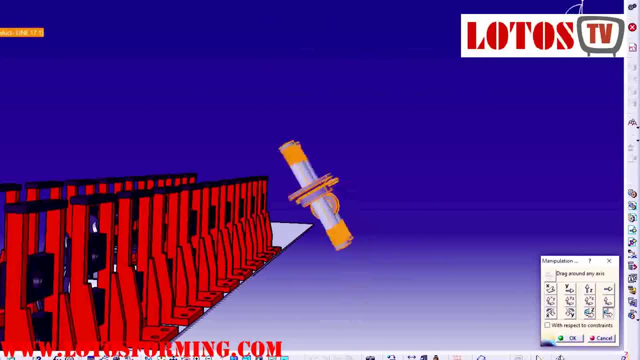 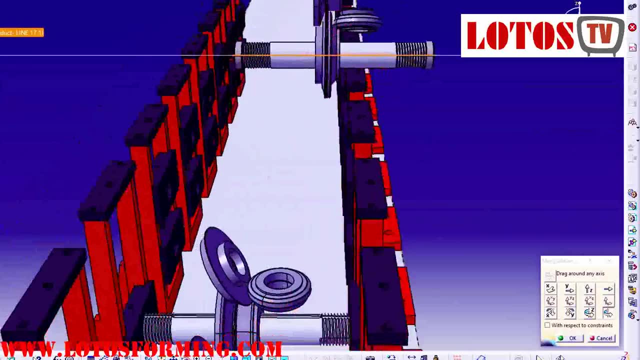 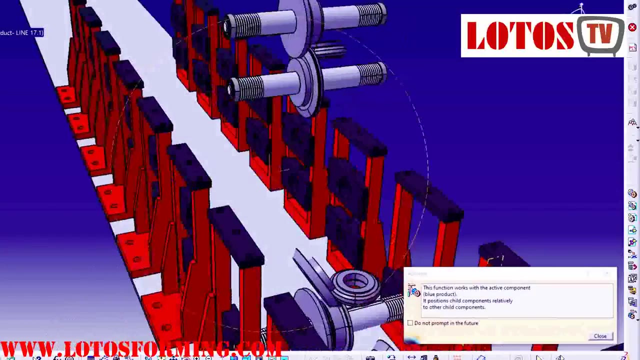 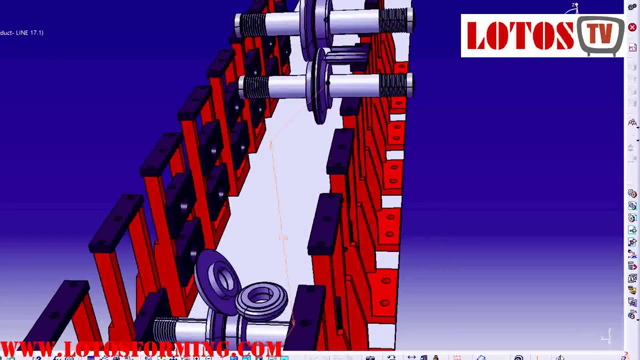 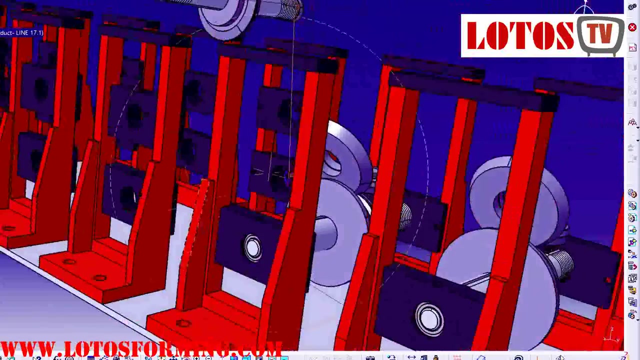 individual plan that we call it casting or standard pillow, related to any thickness or any width. we have a different size standard for pillow. some of them are small, some of them are big, but most of them made by casting method and we have our standard catalog for using that. so a structure of a stand also. we explain to you number six, the. 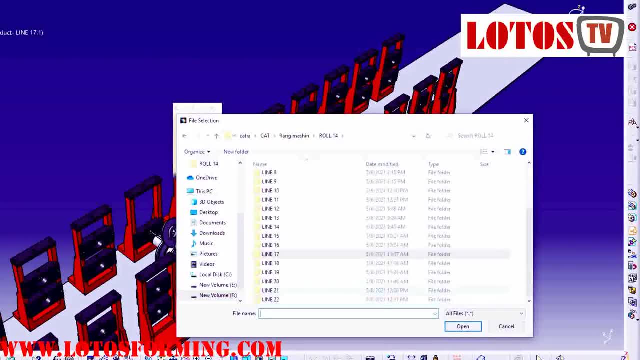 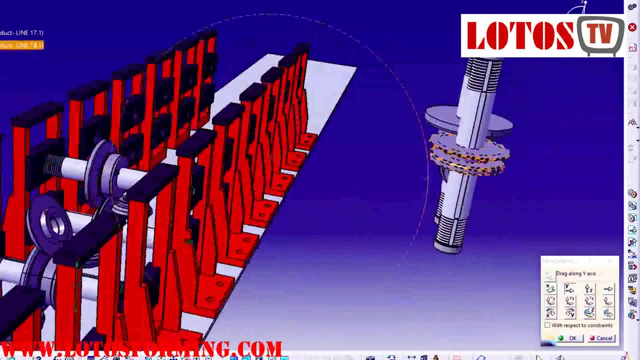 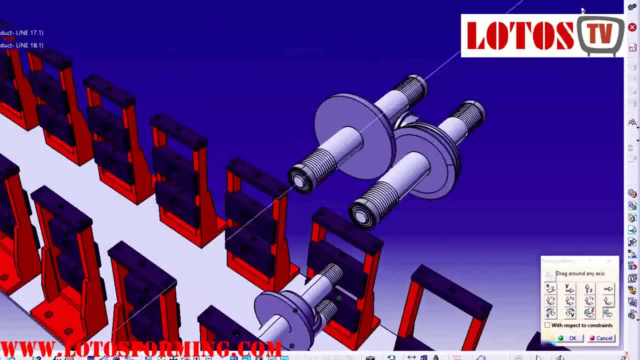 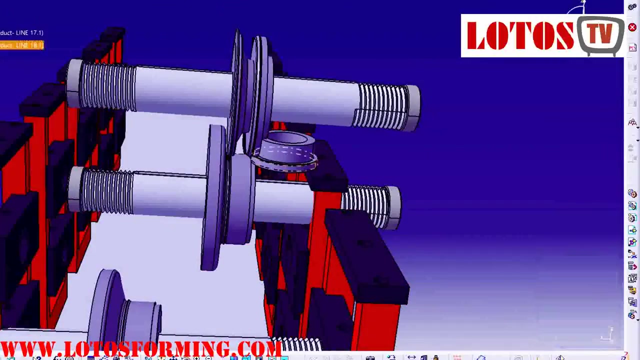 material of rolling tools and this is the main and the most important part. the material of rolling tools related to your raw material that you want to form. we also analyze and choose the different material of roller, so it's really important we use what kind of material for our tools- normally in china. 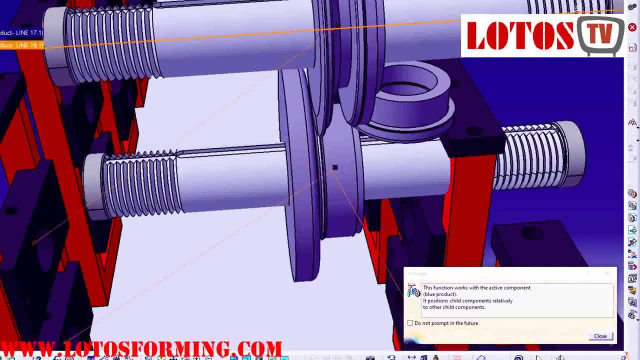 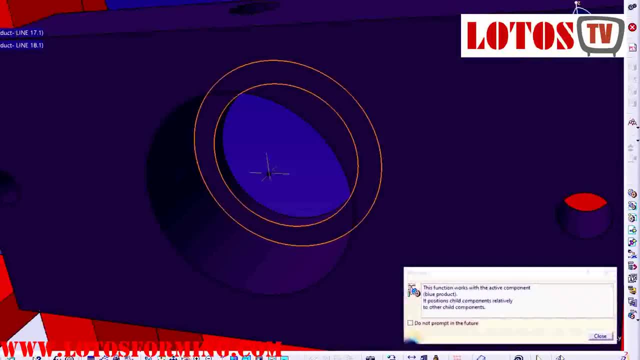 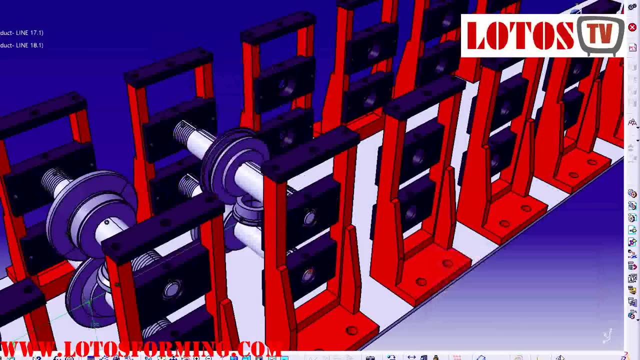 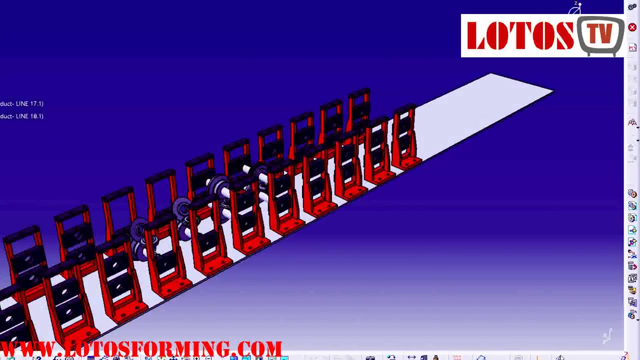 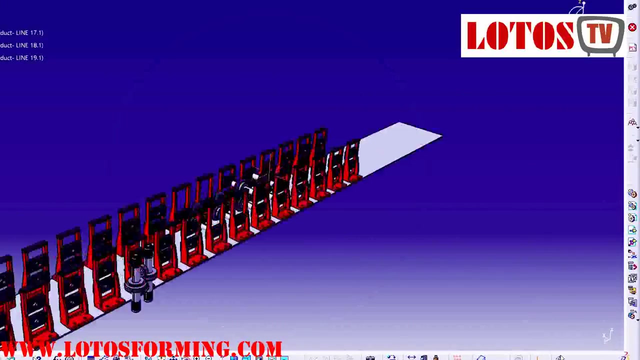 we use gcr 15 or gcr 12, or for chef uses 45 steel, but the most standard way is gcr 15 or gcr 12.. so it's really important what kind of material we use for rolling tools- some of the cheap machine that you can see in the 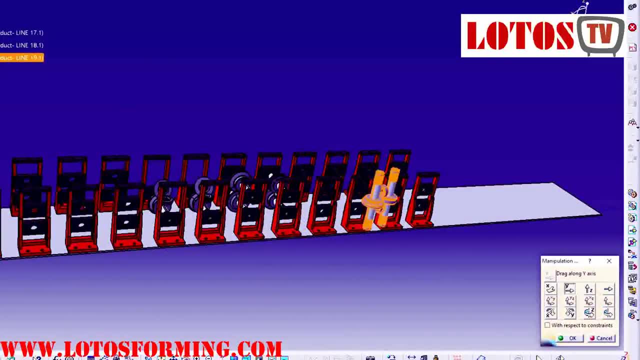 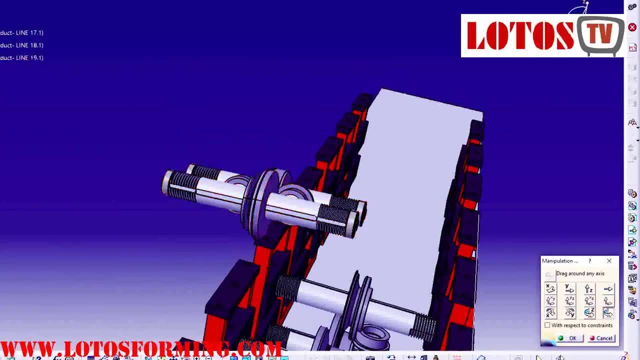 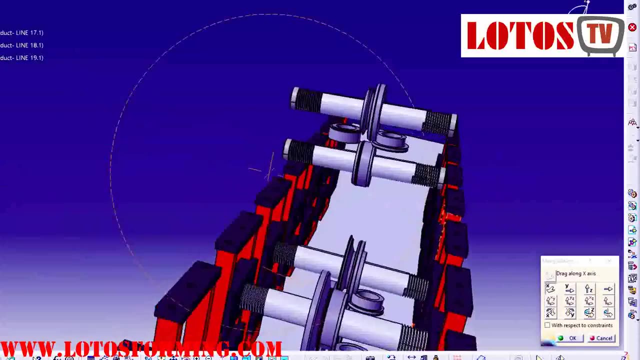 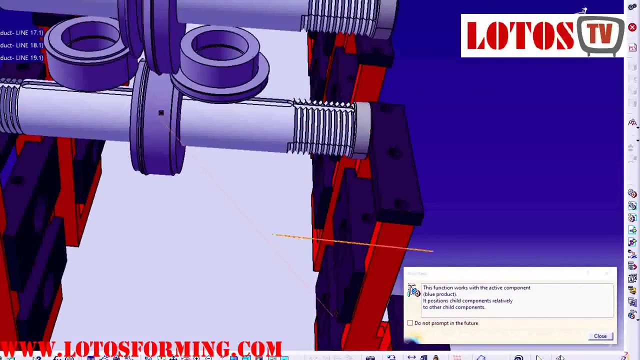 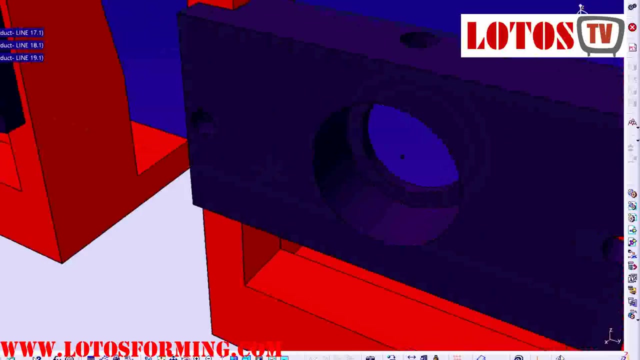 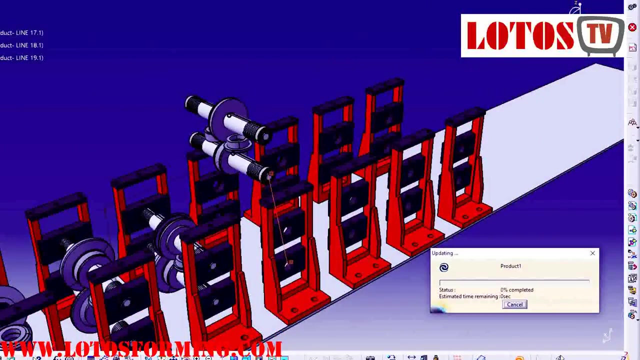 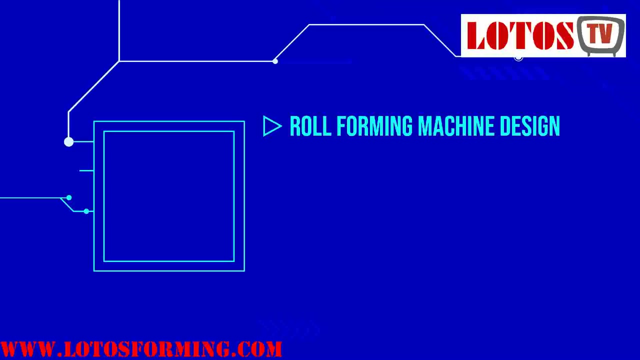 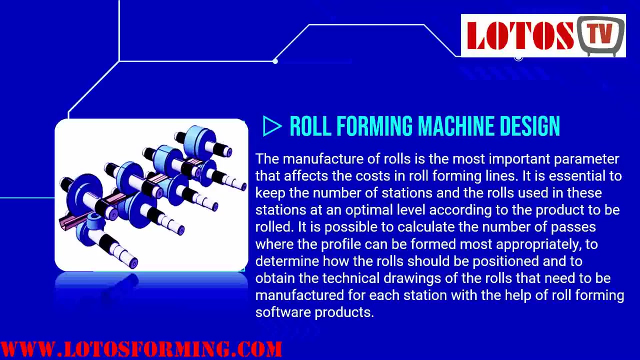 market that we use the lower quality of cheap quality of the material. it will be really short performance period. so we don't offer or we don't suggest you to follow or accept any cheap or forming machine. now I want to explain about reforming machine design. any manufacturer need a really powerful design department for design or forming. 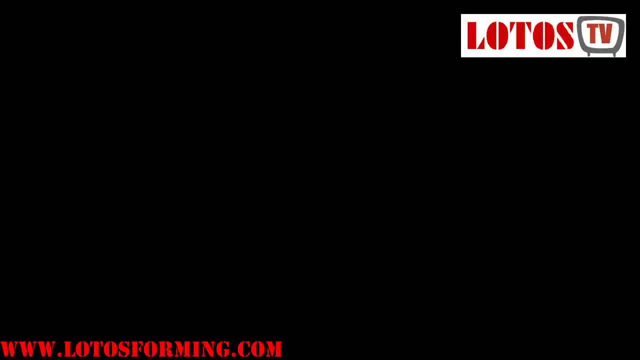 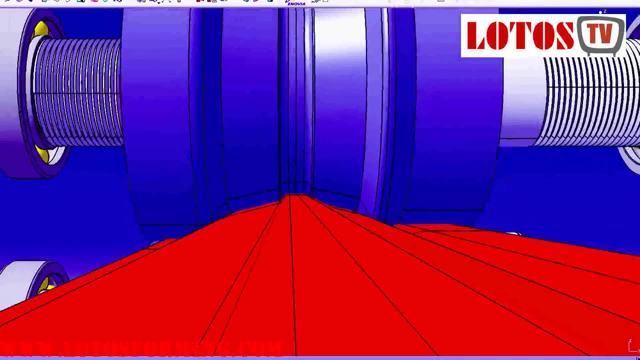 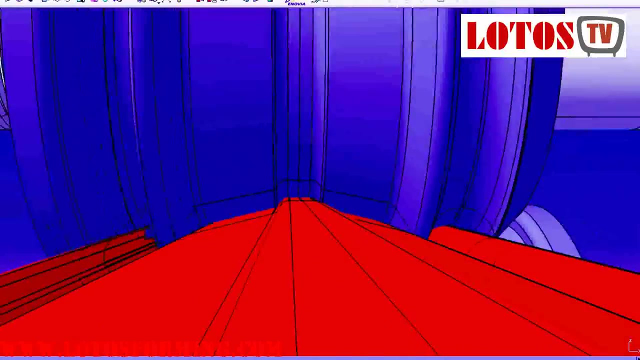 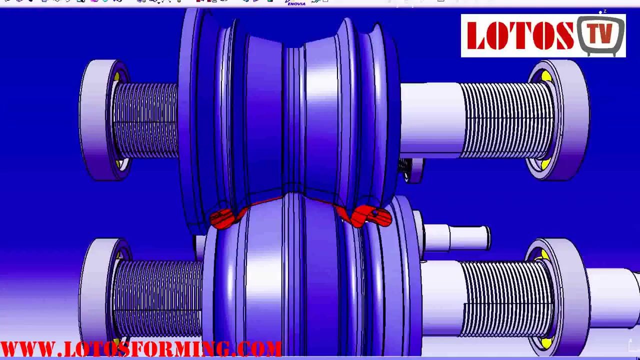 tooling and shaft and it really need a special software like a copra or other software to use an analyst profile and design them, your own forming machine. so the first I, the first and most important part is role forming design to calculate the each amount of the 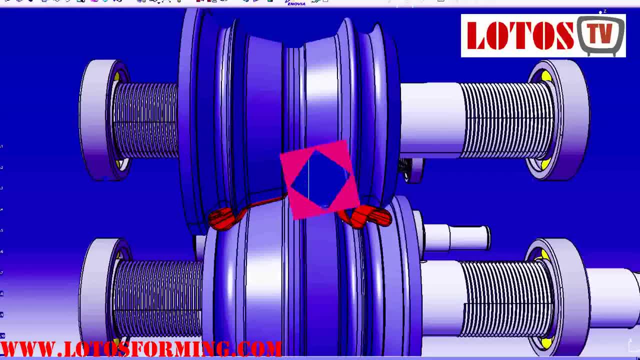 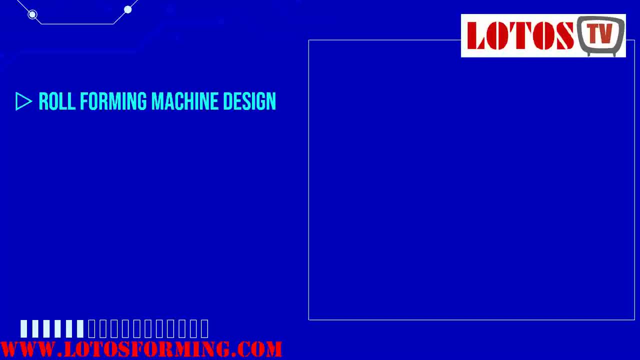 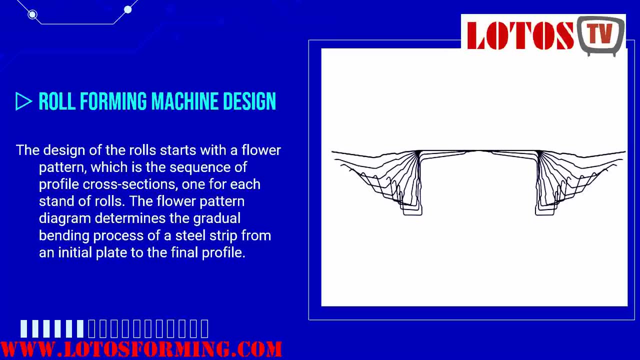 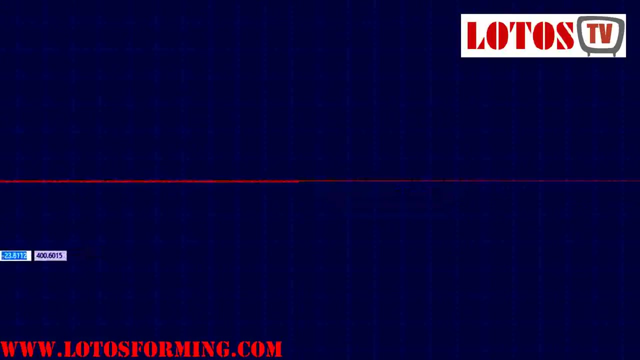 cooling stand and the design for these rollers perform machine design. start by flower pattern, which is there we are always, step by step, the section of profile, how we bend and how many station we need to reach the final result. so, as you can see here, here is the flower pattern for any profile cross. 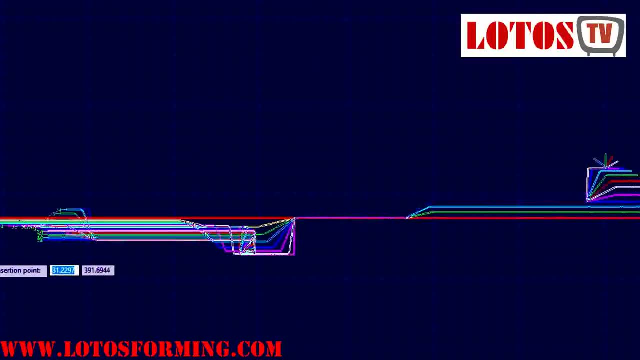 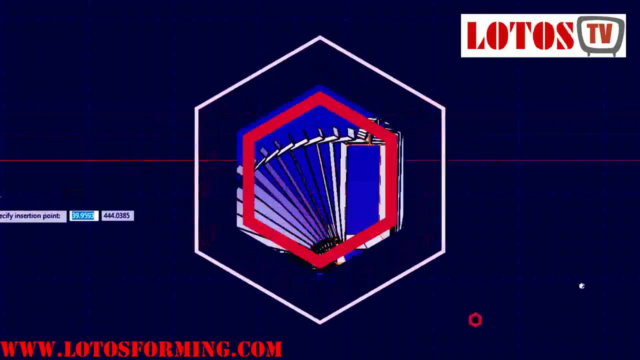 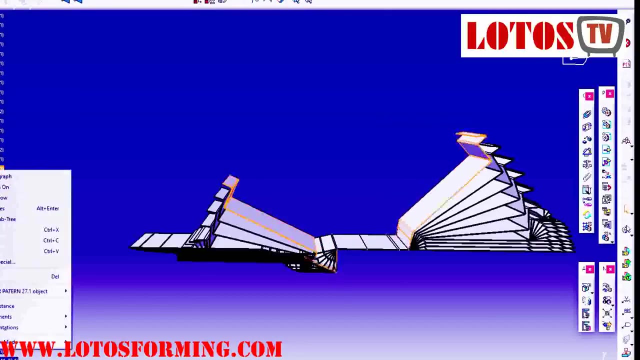 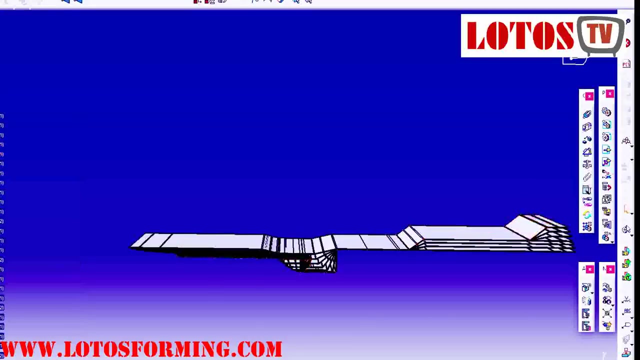 section that show you how many stands or how many tooling, a standard need to show you one really complicated role forming machine that has almost 44 tooling a stand. here I show you the flower pattern one by one that you can see and you can understand what we call flower pattern. based on these flower pattern, we go to design the 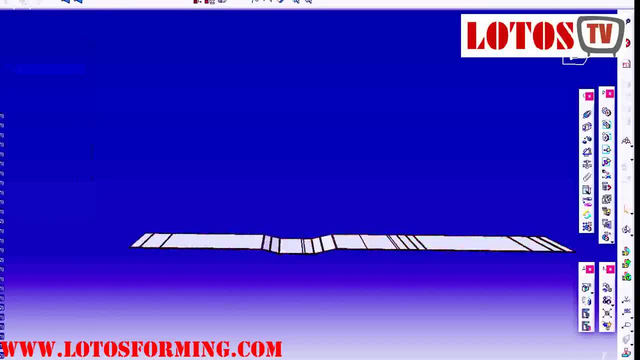 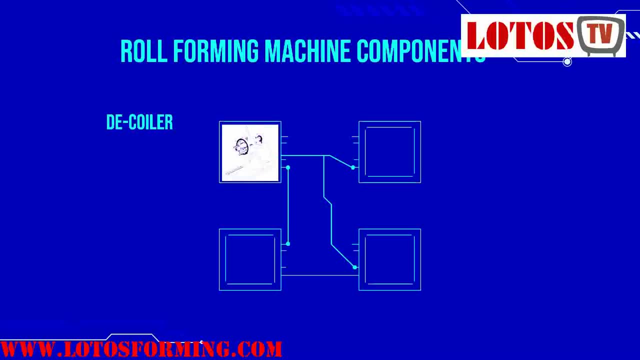 roller and shaft and any part of machine. now we talk for all forming machine components. first component is the coiler for all forming machine to load raw material, coil into that and start to feed the material. it's a second. there is feeding roller and it's tightening for leveling and feeding the material into. 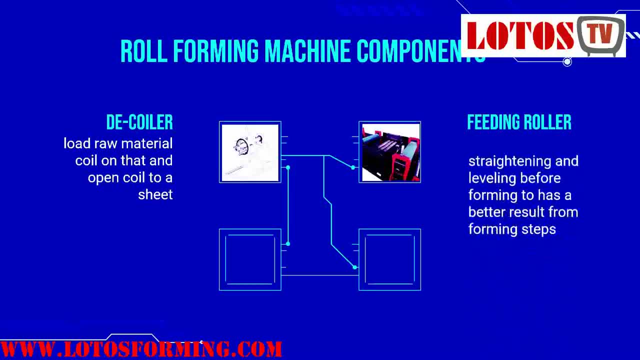 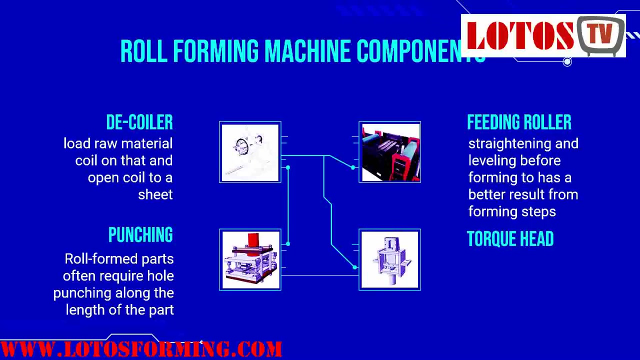 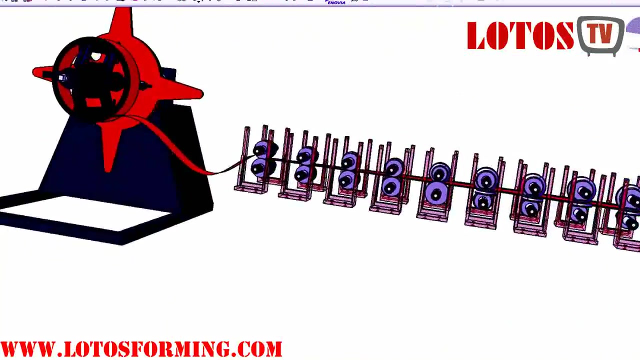 the tooling stand. third is forming stands and fourth is punching for any punch, any hole or any notch related to your design and requirement. then we go to torque head and final cutting. so this is some general view I show you. here is the coiler, as you can see. then we go to 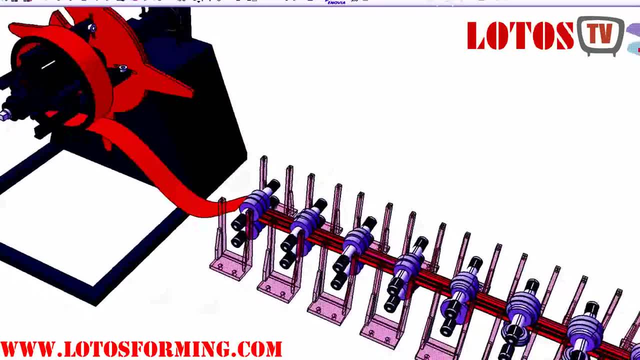 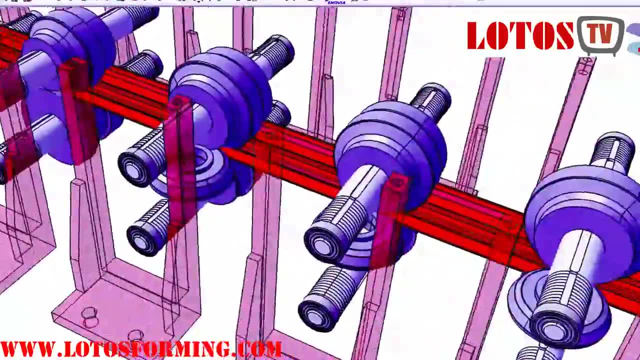 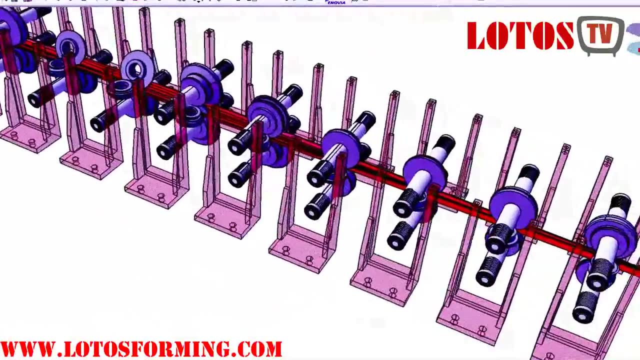 the roll forming stands, shaft roller, one by one. you can see this is some general view for one of our forming machine, if I'm sure it should be some flange profile. so here's the punching during the forming. some of our punching will be before forming, during the 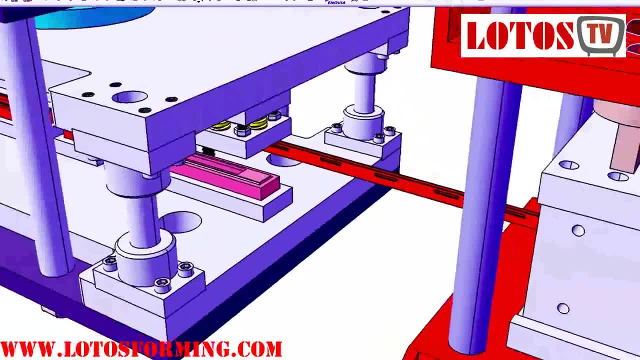 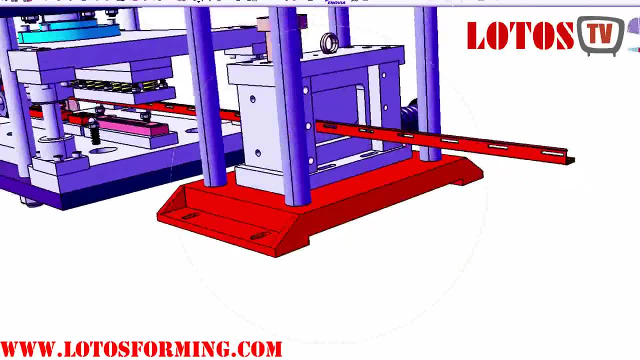 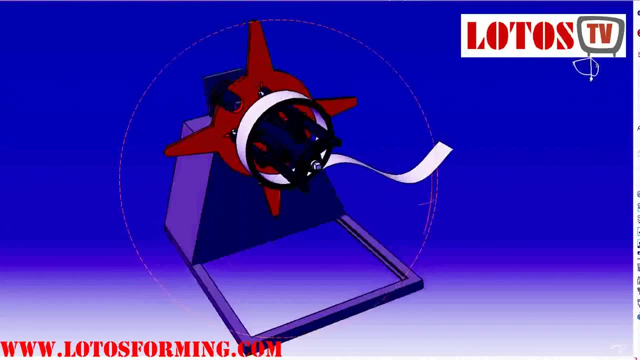 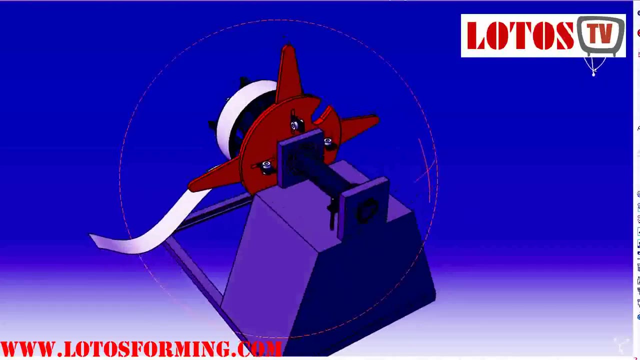 forming, during the forming or after punching. we call it final punching. and here is the cutting before out the taper. we cut it to lengths in the plc. here again the coiler. I'm turning around to show you what's the part and how simple it is. but it's really. 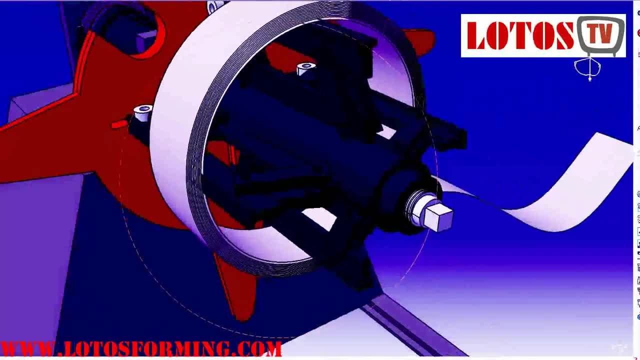 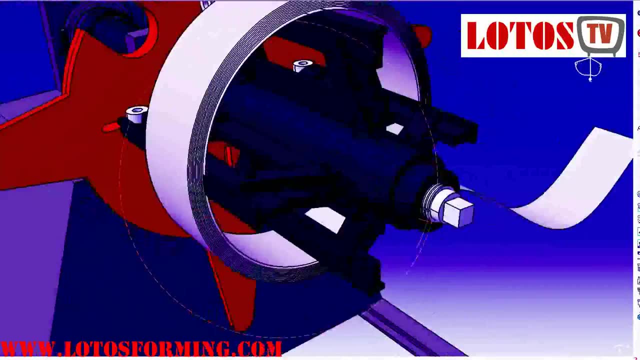 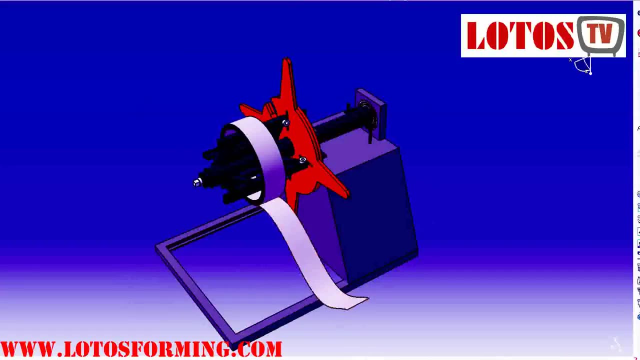 useful for any roll forming machines. it has a forearm and it's really work easy. here's the punching. you can call it peeling punching, because you can see the material is flat. here's the tuna coin. so if you want to take a look at tusORD machine, she gave us this. 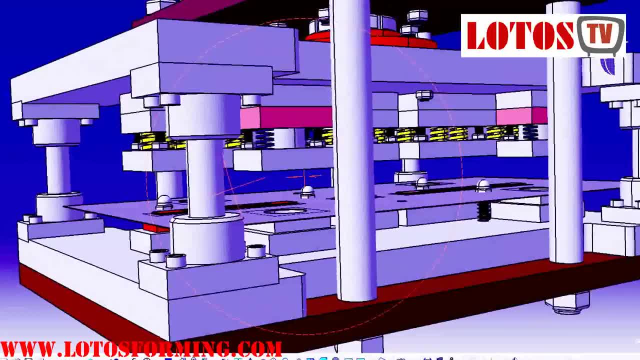 little one here, and before forming and before go to the tunning, a stand, we make a hole on that, we make a notch on that toian name from it. so it's punching, the zoom soumtion and we'reくあり awesome, the hole on the die. so I mean, this is like a ring. don't cover it or not. I'm going to. 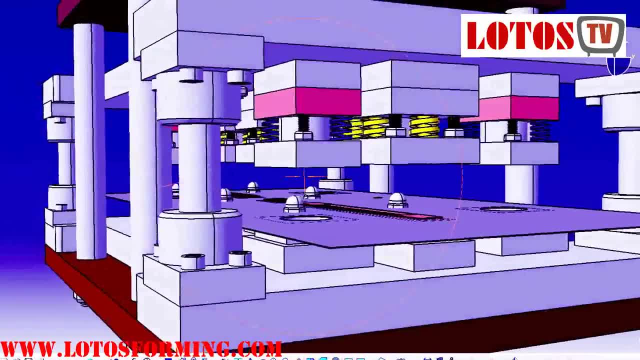 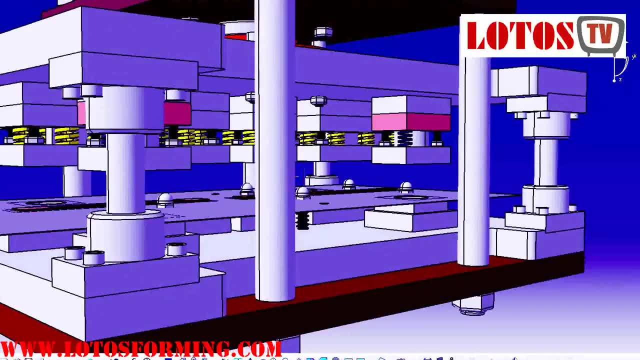 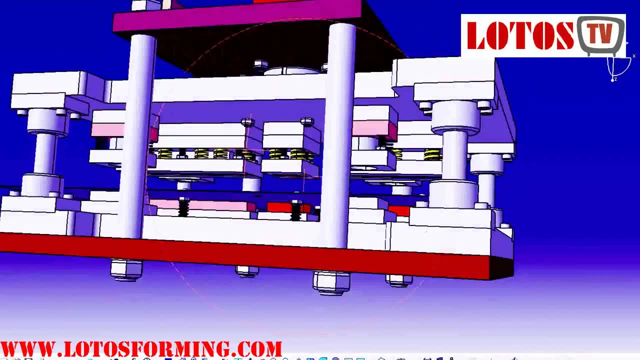 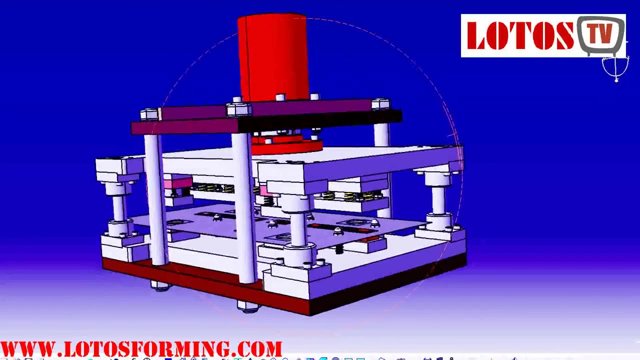 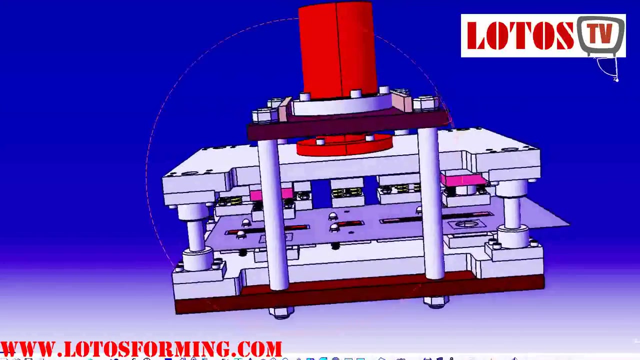 be the same way, like I did before. so there's a hole before and I made winch to only connect before forming. turning around for you to show you design of this punching. this is for door frame for or one of customer in Middle East. we designed this pre punching unit. 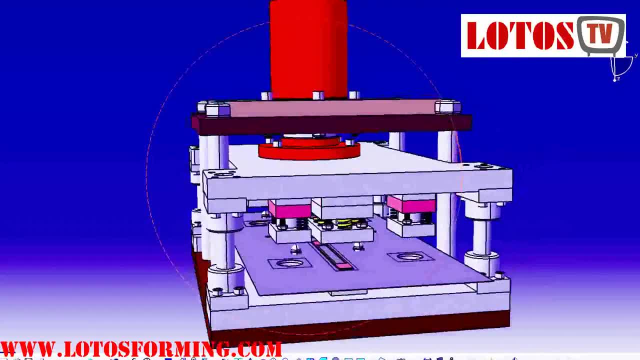 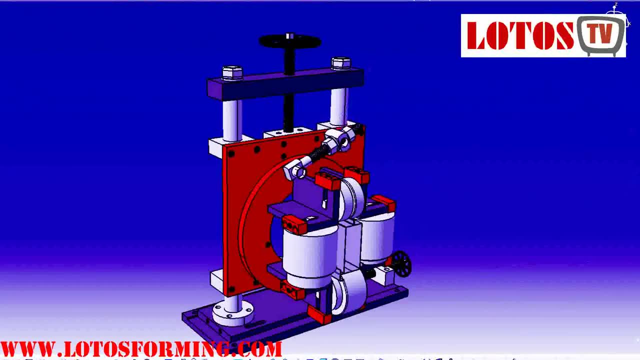 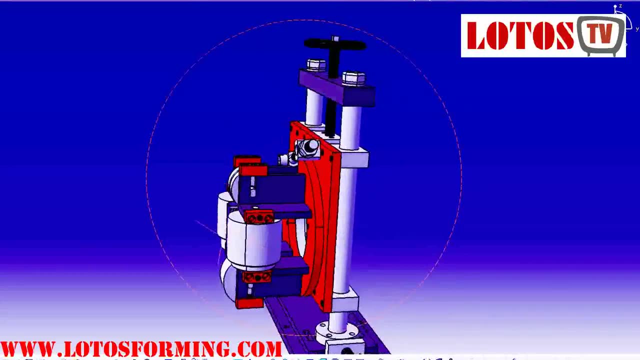 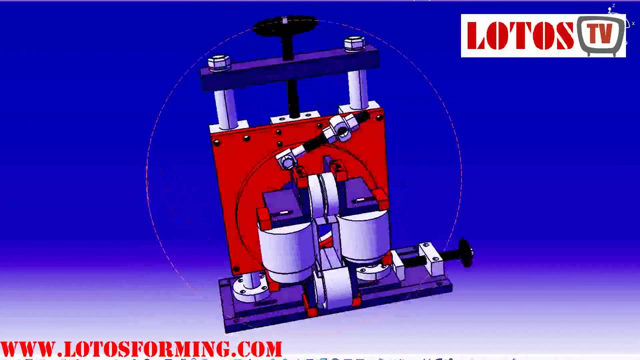 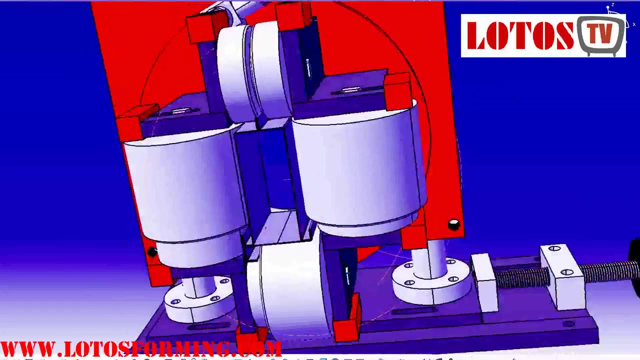 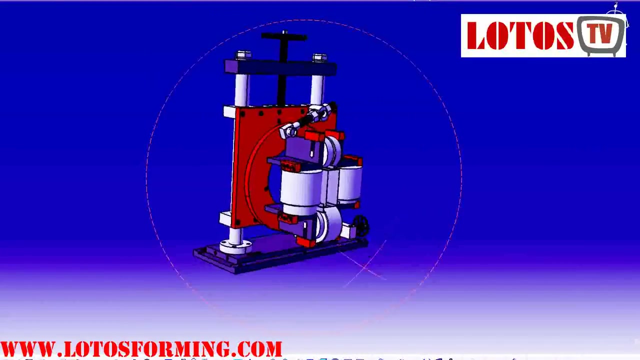 later I will show you the complete line of this machine. we call it pre punching and here is the torque head. this is really important for any roll forming machine. for a straightening bow twist, we use this torch it. it can be moved up down, twist left and right for axis movement and it's really 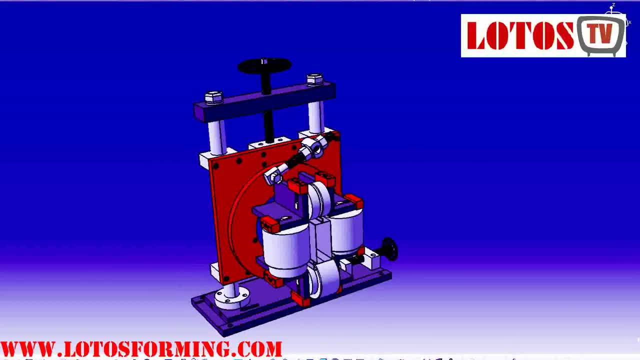 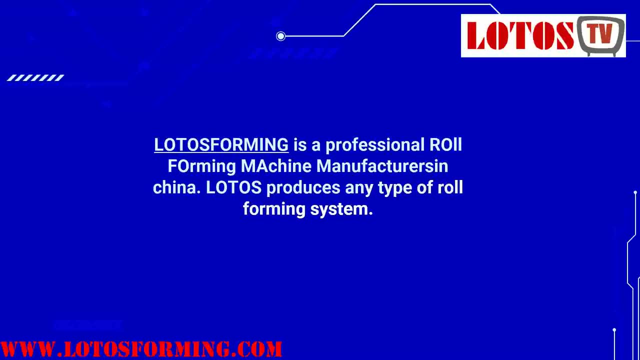 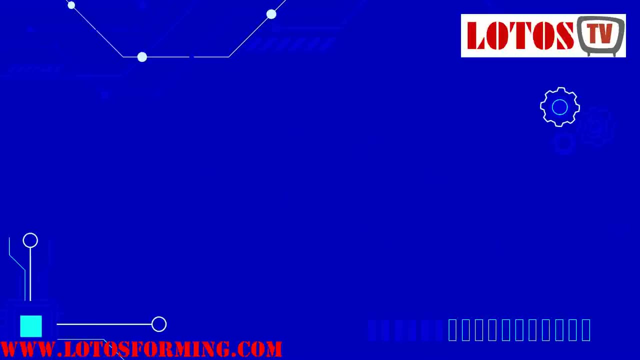 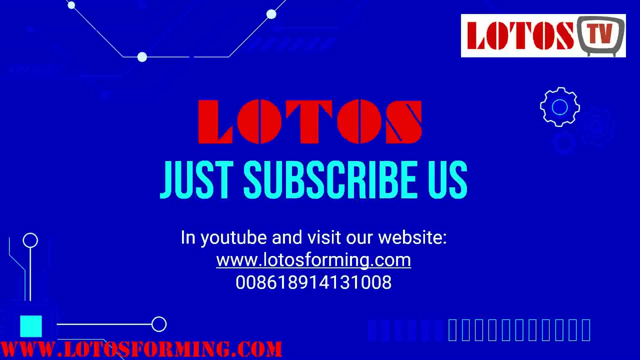 necessary for any roll forming machine to get a final result. so don't forget about Lotus and hold on to it until you get the final result you enjoy about this video. for any question or any requirement, feel free to contact us. we are from Lotus. just subscribe us and follow us. thank you, bye. you.